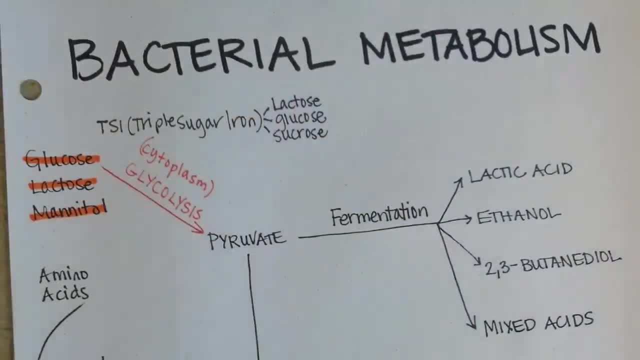 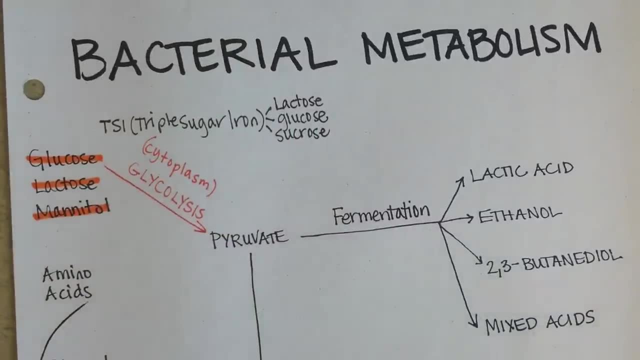 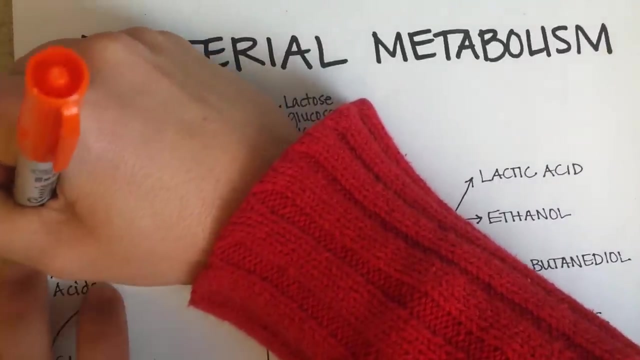 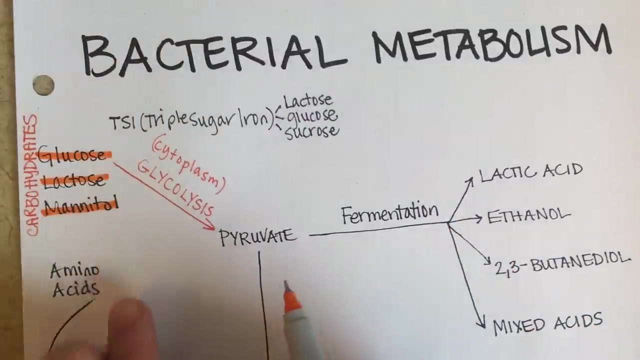 Sucrose is a glucose connected together with a fructose, so if they can't break those two apart, then they're not positive for sucrose metabolism. these would all be classified generically as carbohydrates. so we'll be studying the ability of different bacteria to metabolize different kinds of sugars and that process. 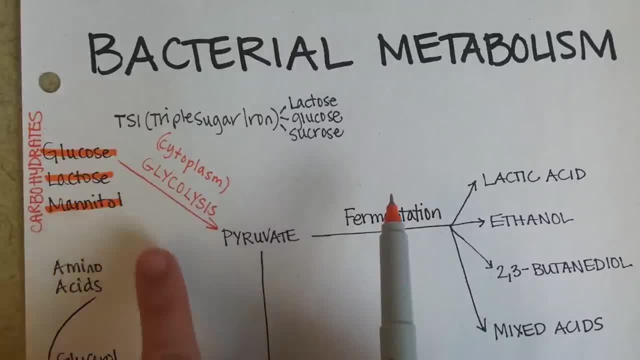 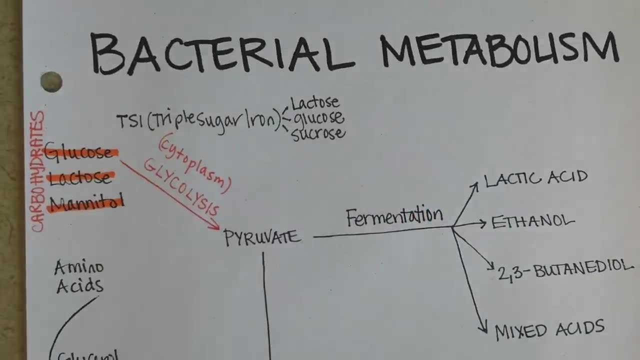 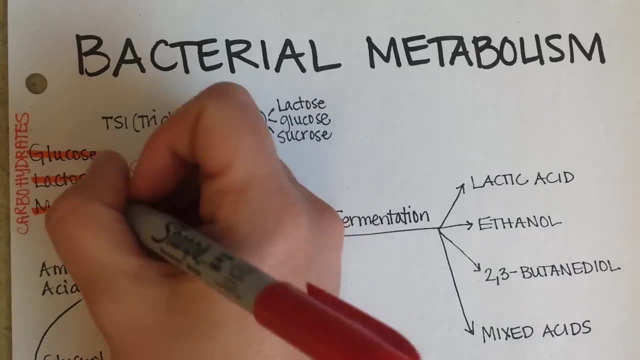 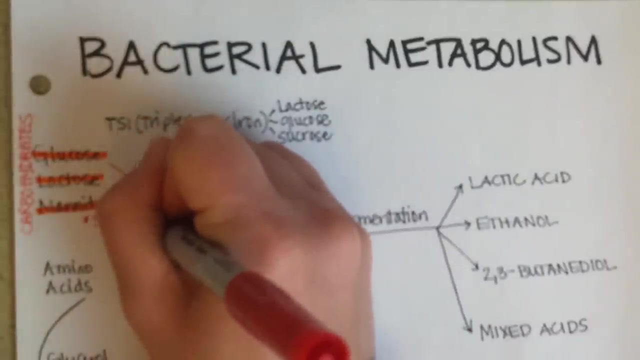 of glycolysis is converting glucose, lactose, mannitol, variety of other sugars, to pyruvate. mannitol, like I said, is special in that only a few bacteria that we study and that are medically significant can convert it to pyruvate. one is staph aureus, one is enterococcus. 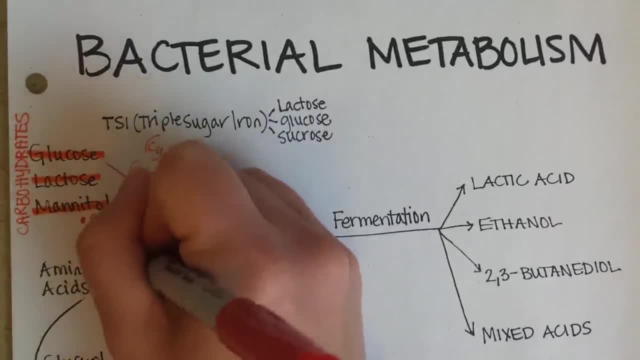 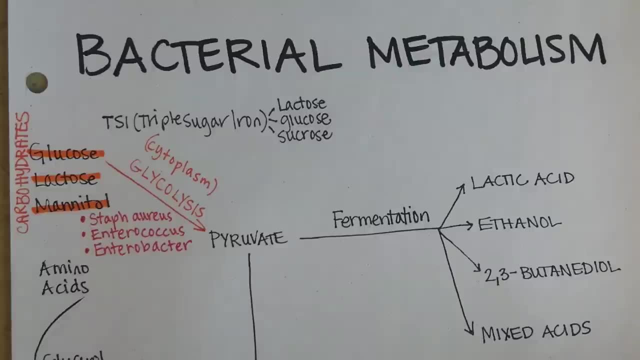 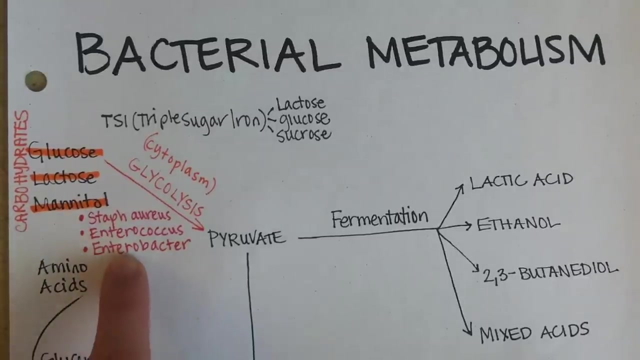 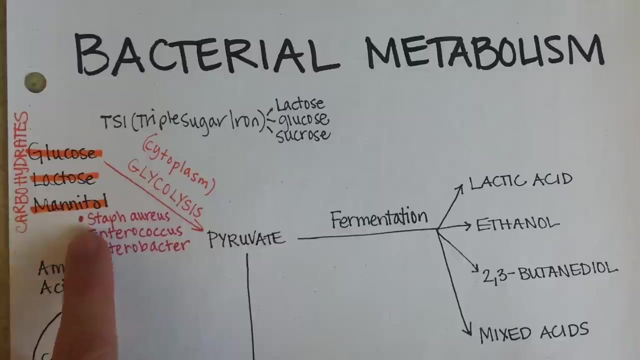 and one is enterobacter. so there's a test that we'll do in lab called the MSA or mannitol salt auger test, and these three genre of bacteria are able to ferment mannitol to make a little bit of ATP, so they actually turn the. 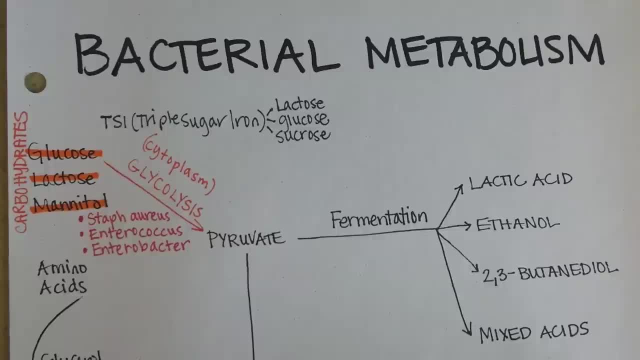 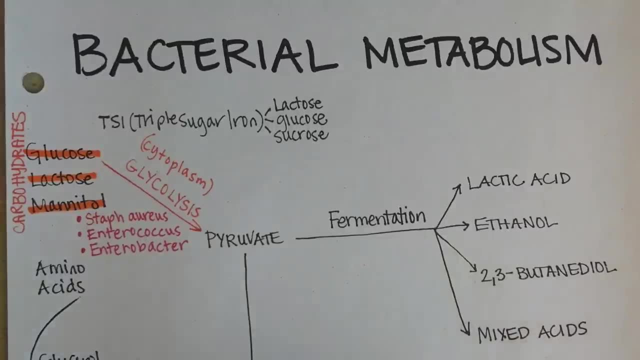 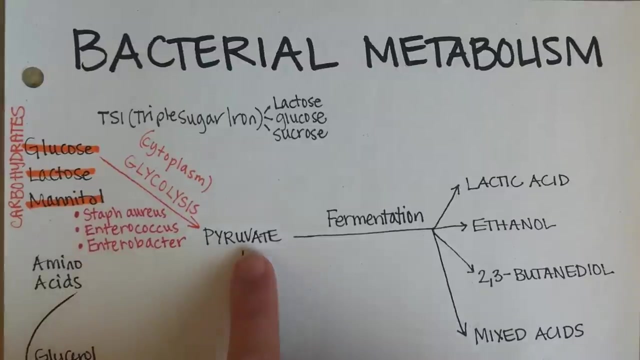 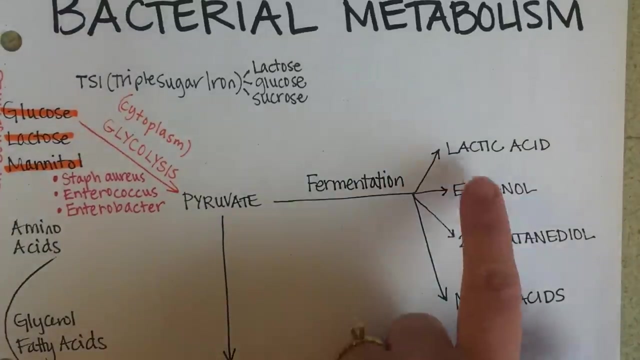 petri plate a yellow color because of that positive result and that will become important when you're trying to identify bacteria. okay, so then, after glycolysis comes the next process: fermentation. and fermentation is converting pyruvate into one of these four products, so lactic acid, ethanol, or alcohol 2,3-butanidiol. 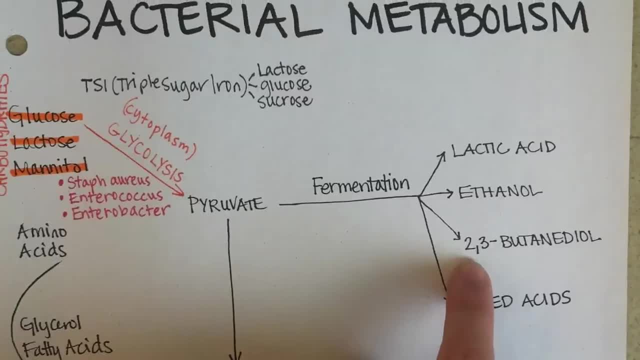 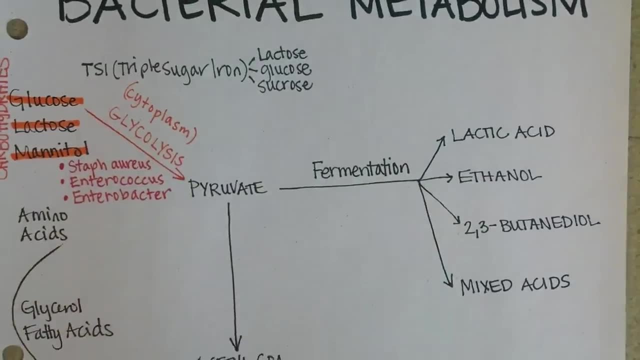 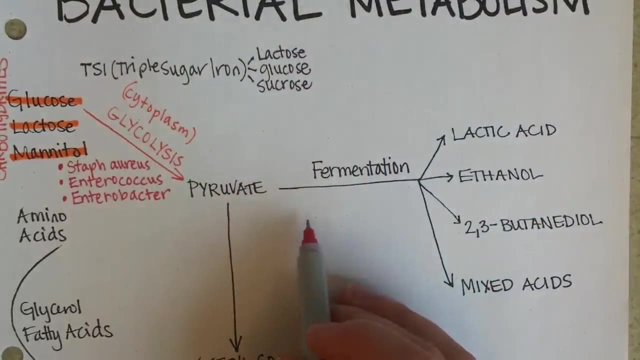 which is another kind of alcohol, but that one is not something you would drink- and then mixed acids. they can kind of make a little bit of all of these things, and it depends on which enzymes the bacteria have, which of these they can do. so actually I'm not going to. 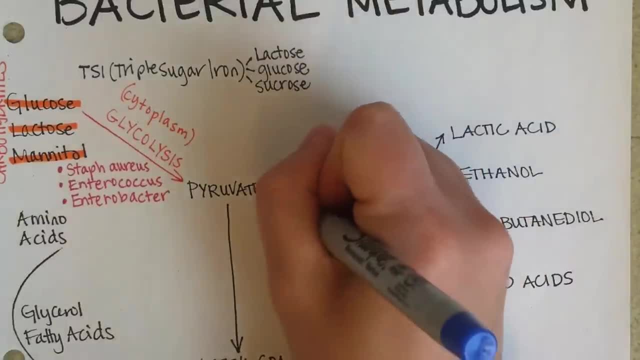 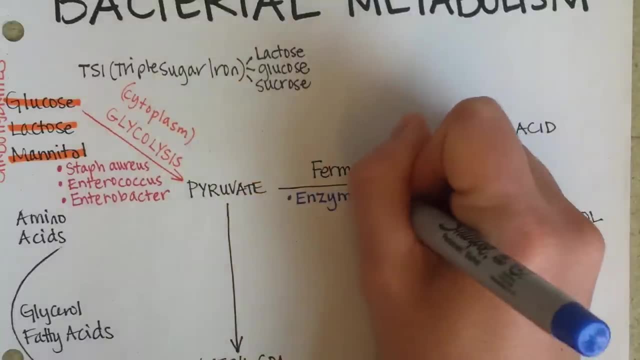 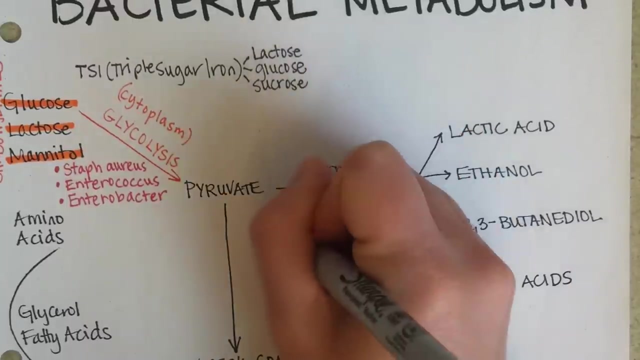 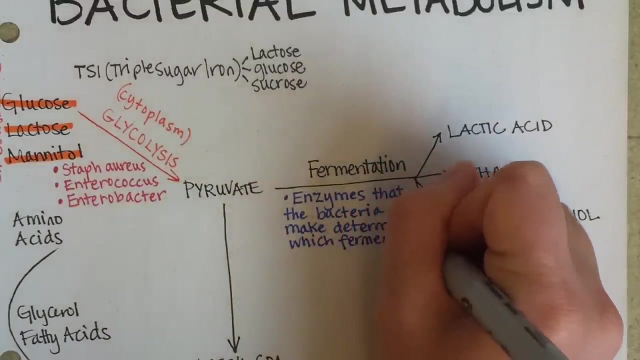 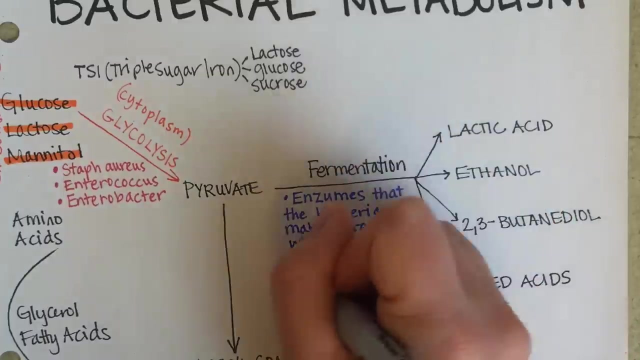 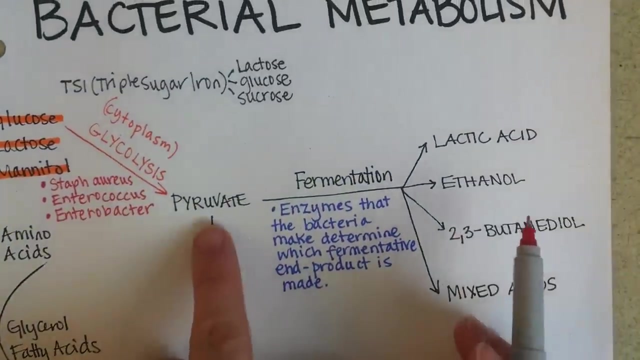 use red. right there, I'm going to use blue. a key point is enzymes. I do it 1 Ensign. so, for example, lactobacillus makes enzymes that when pyre calling tree makes, but that when pyre calling is fermented it converts it into lactic acid. 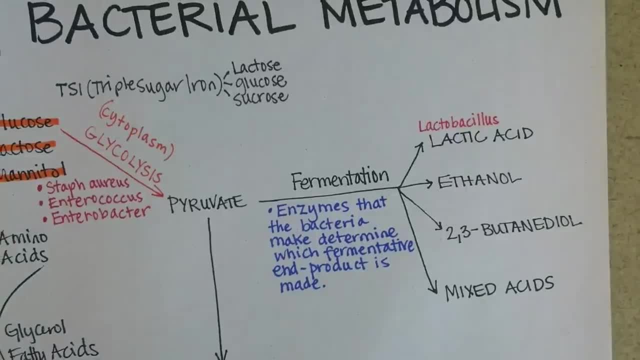 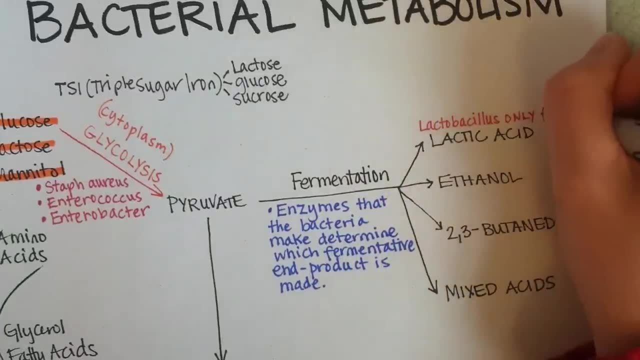 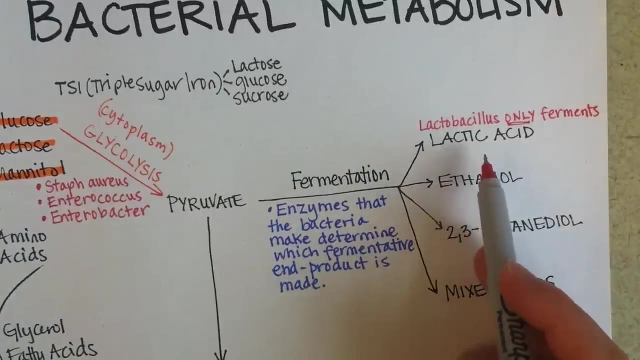 Interestingly, lactobacillus is a bacteria that doesn't have an electron transport chain. It only is able to ferment. That's all it can do to make ATP And its end product being lactic acid is very sour And its end product being lactic acid is very sour. 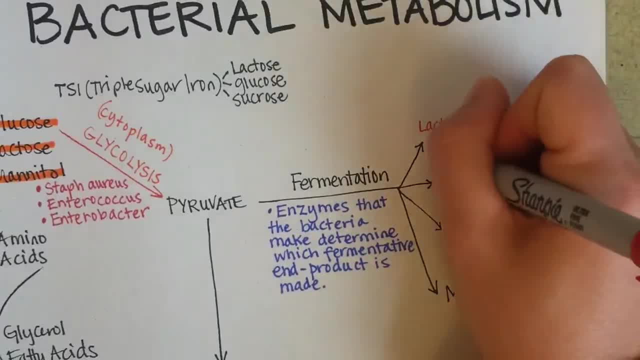 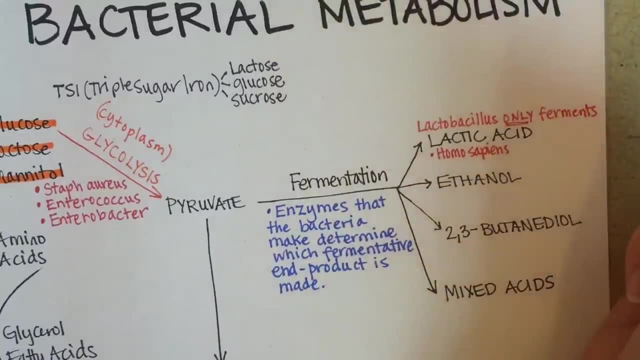 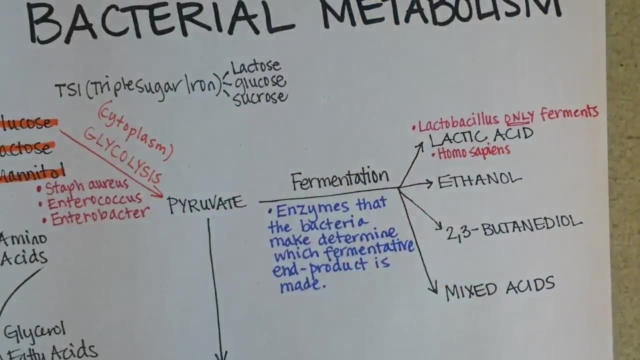 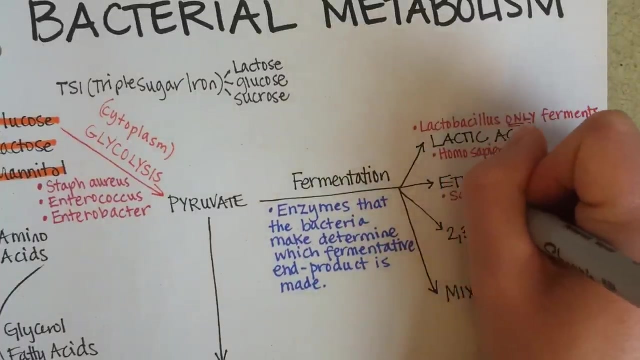 We're also able to do this, so homo sapiens. So we produce lactic acid when we don't have oxygen available for ATP production, and so does the bacteria lactobacillus. Ethanol is produced by saccharomyces. remember that stands for sugar fungus. 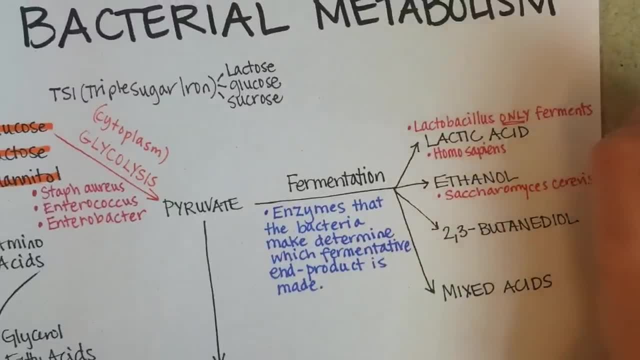 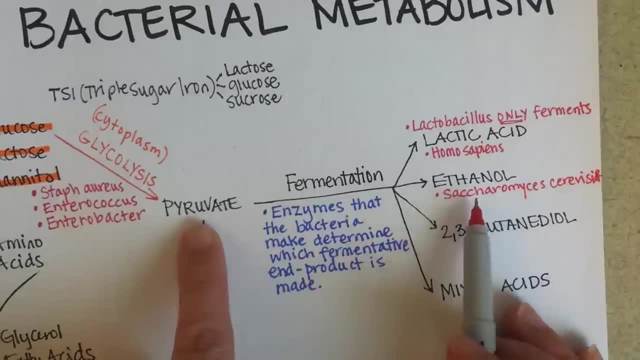 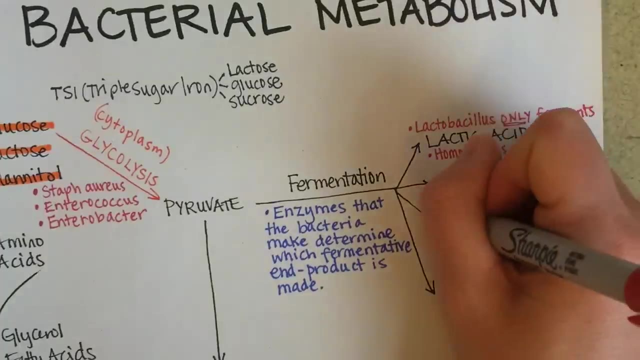 cerevisiae beer, So saccharomyces cerevisiae. That ferments pyruvate to ethanol and that's where we're able to get wine, beer and hard liquor. Interestingly, candida also does this. It's another kind of. 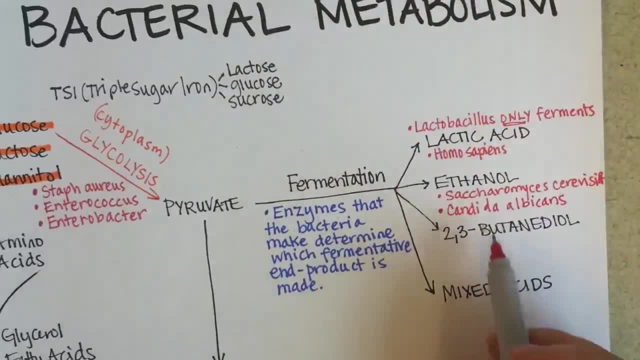 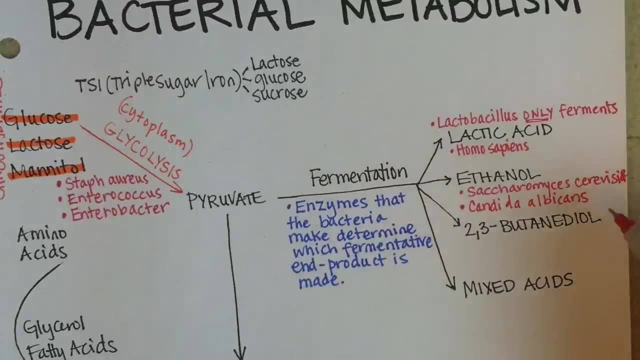 fungus. but instead of being used in the food industry, candida albicans can overgrow in our gut or in a yeast infection, And in fact there have been reported cases of someone with such a bad candida infection in their intestines that they start to 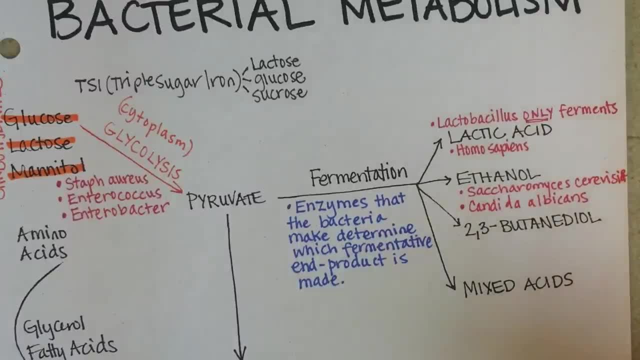 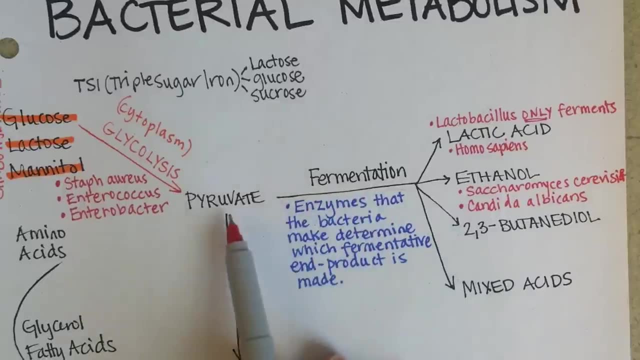 behave as if they are a little bit drunk. How clinically common this is, I doubt, but I have heard of it. Okay, so then, 2,3-butanediol is an alcohol that is produced by a particular bacteria called enterobacter. Now, in the real world, this one doesn't have a whole lot of interesting. 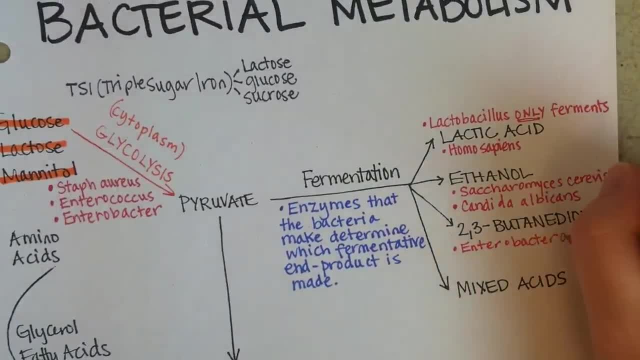 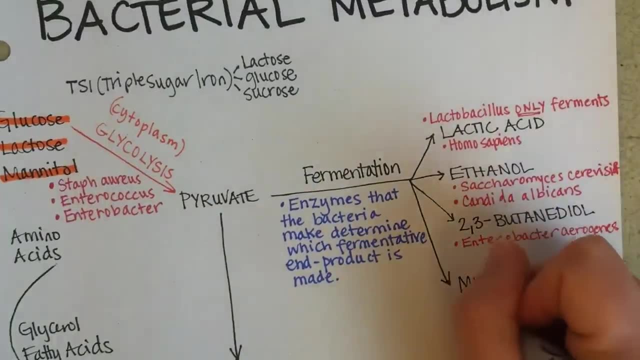 application, but it does matter in the lab When you are trying to figure out whether the unknown bacteria you have is enterobacter or E coli. So E coli produces mixed acids and enterobacter produces a pure product of 2,3-butanediol. 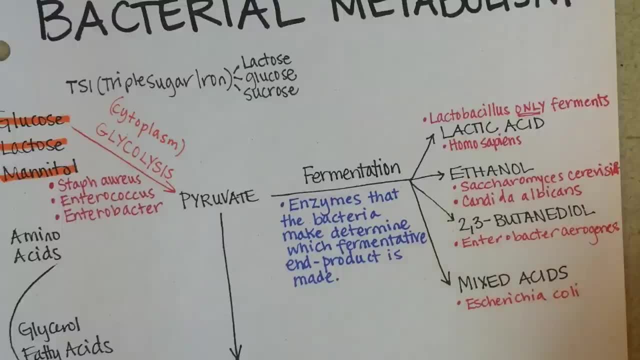 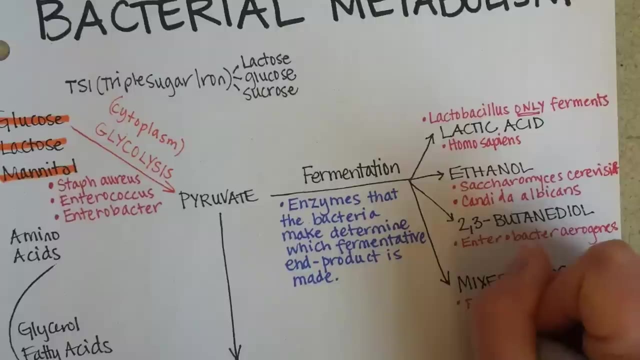 These are really similar in other areas in lab, and so there will be a test you do, called the MRVP test, that can help you tell these two apart. We can use our black pen, So there is a test called methyl red or MR. 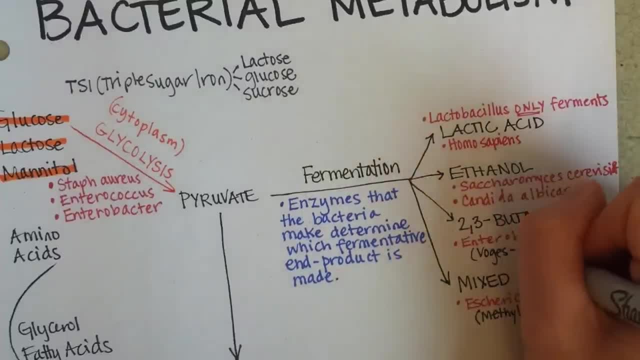 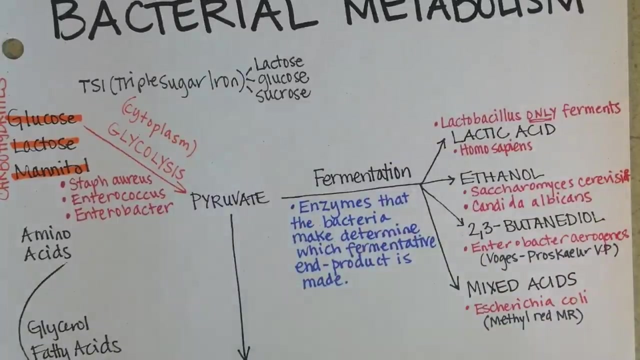 and then there is one called the Vogues-Roscower, or VP, and then if you put those two tests together, we call it the MRVP test, in order to differentiate between E coli and enterobacter. Also, I am going to put in other 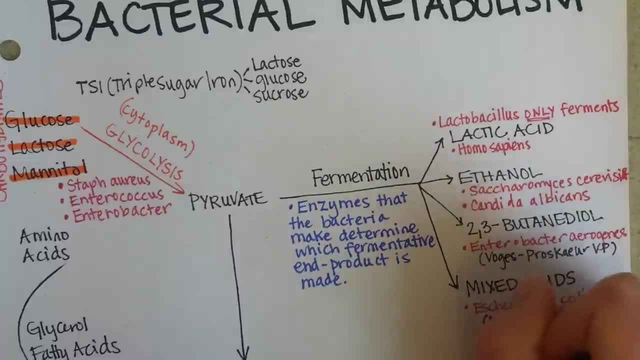 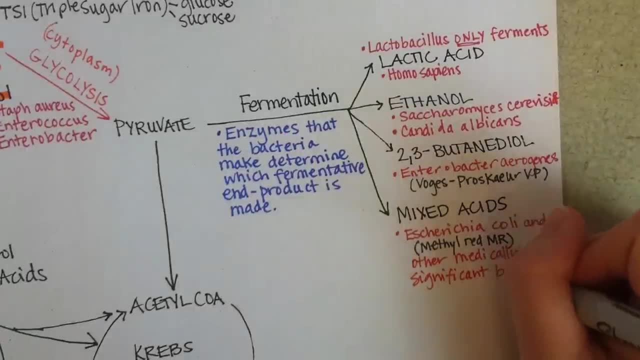 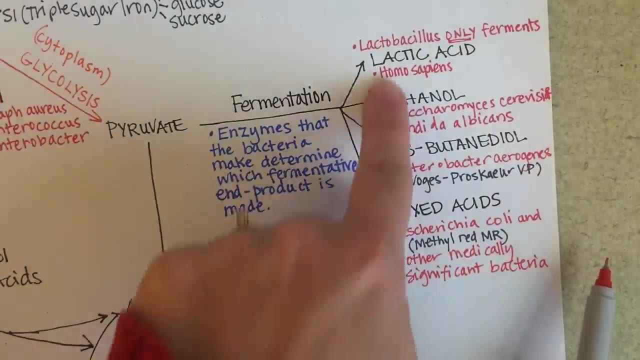 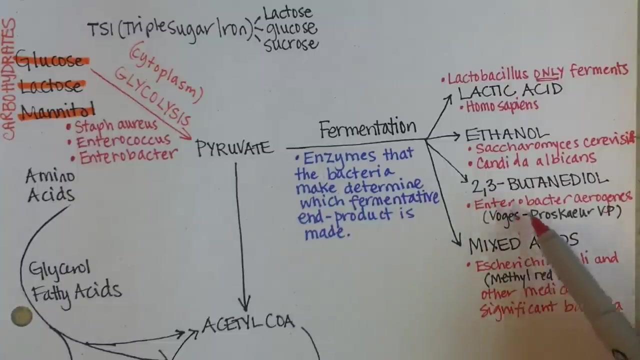 medically significant bacteria. There is actually lots of bacteria that produce mixed products because they are more versatile. right, If you can give them pyruvate and they can produce a little bit of all of these things, or a variety of different acids, then they are going to be more versatile than, say, for example, enterobacter. 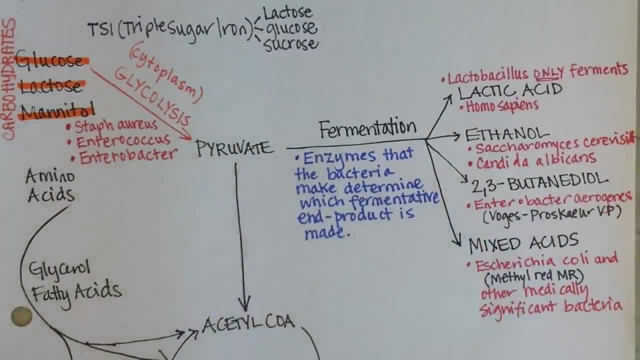 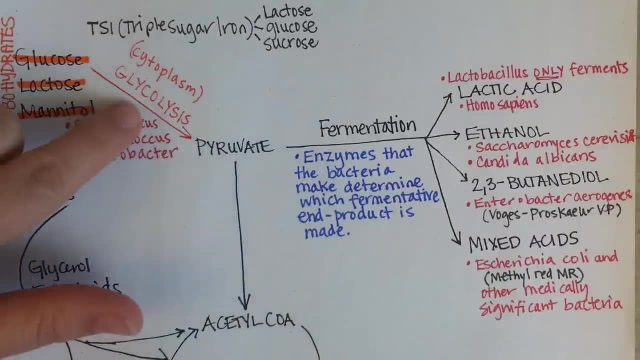 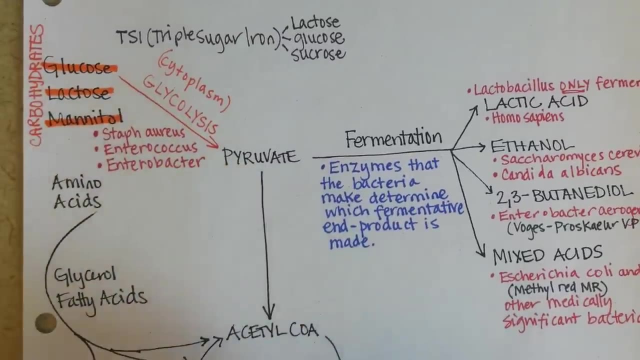 which is only able to ferment pyruvate into one end product. Okay, so recap a little bit. Glycolysis occurs in the cytoplasm of all living things, and it is the process of converting glucose into pyruvate Bacteria are able to take. 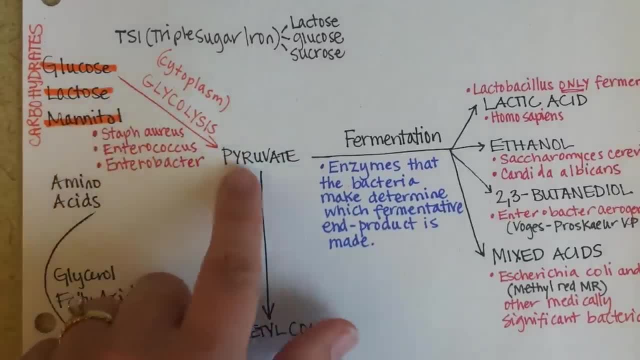 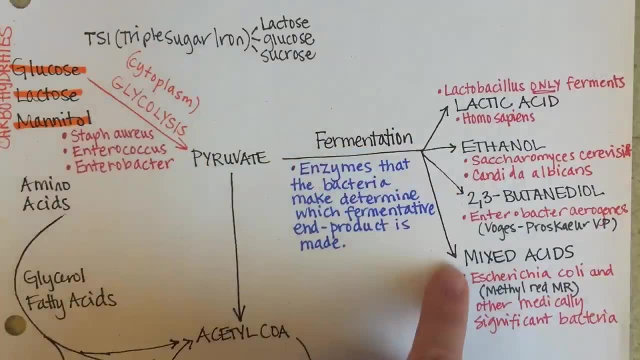 a few other products and also, one way or another, get them converted to pyruvate. So that is the first process, And then pyruvate can be fermented into one of these variety of products, and most bacteria are able to ferment into pyruvate. 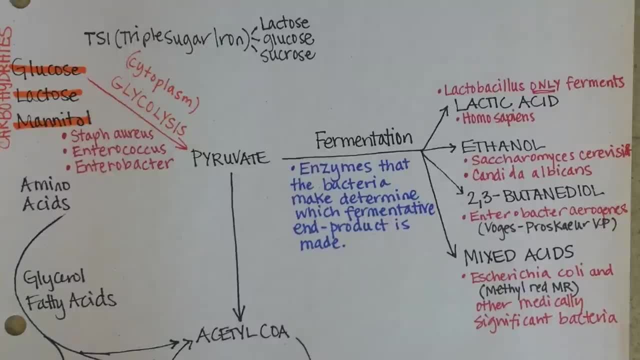 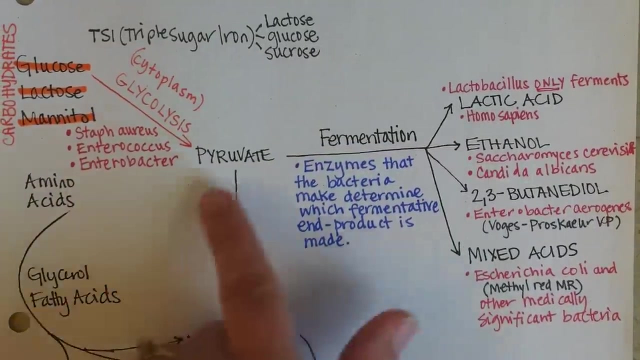 There are a couple bacteria that are not able to ferment. Pseudomonas aeruginosa, supposedly, is one of those, although I have heard clinically that they are even finding that that occasionally is able to ferment. So most bacteria can ferment And then, if oxygen, 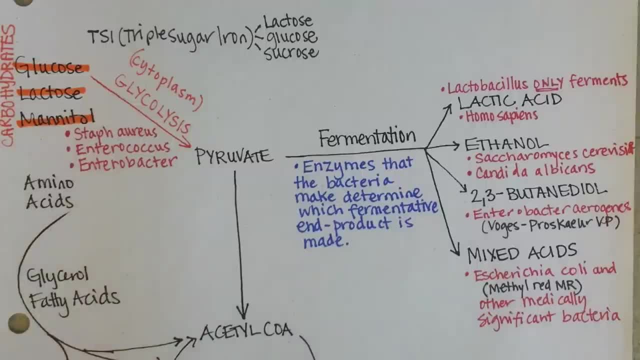 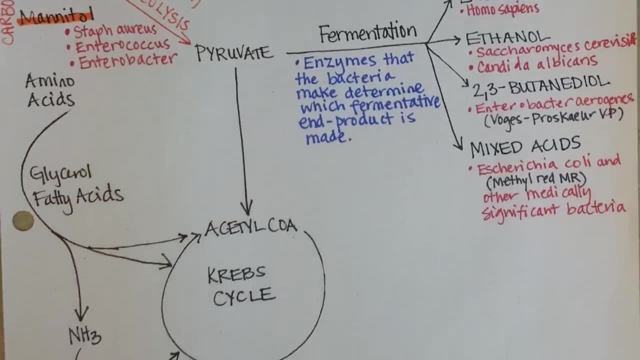 or another very strong electronegative element is available, pyruvate can also then enter the cross section of the body. So that is the first process. Krebs cycle, or the citric acid cycle is the other name for it. 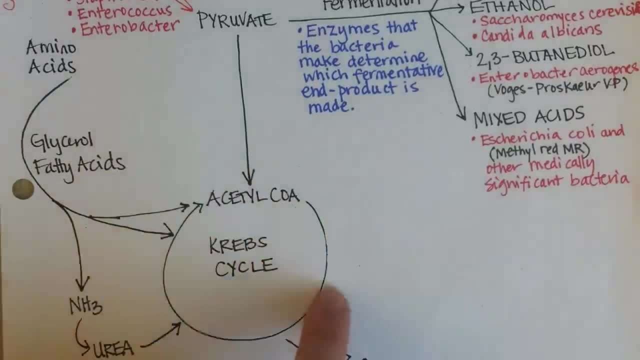 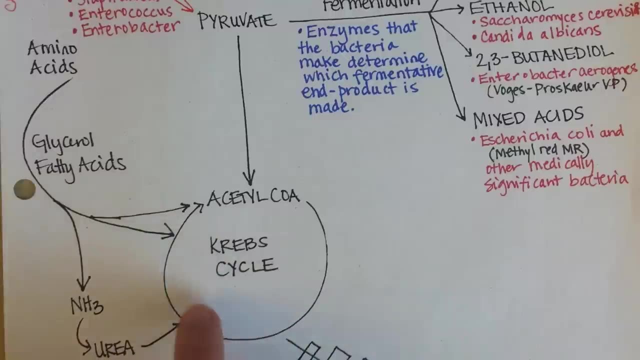 And the reason it is called the citric acid cycle has to do with the recycling of a citric acid compound. So this is the circle represents enzyme changed into enzyme, changed into enzyme, and so on in this repeating cycle, And then ATP. 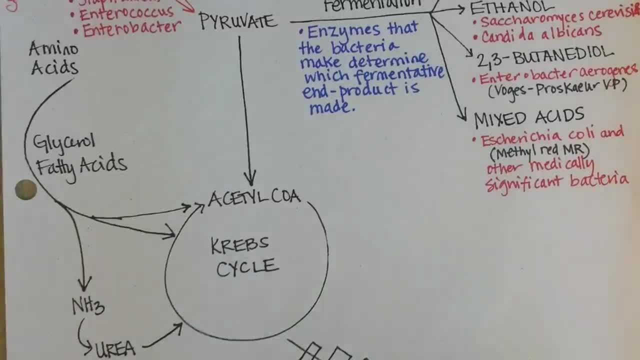 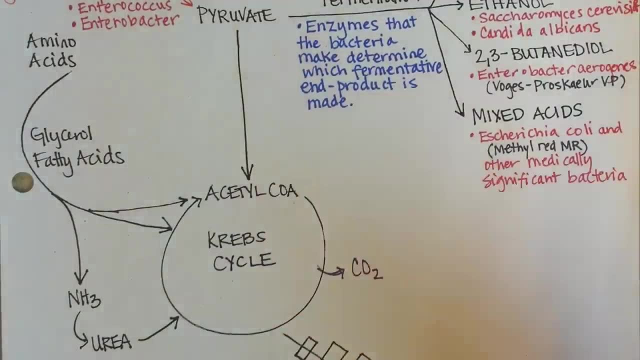 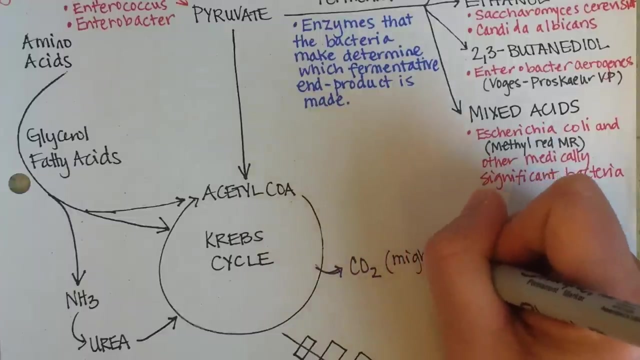 excuse me, ATP is produced a little bit and also some carbon dioxide, So you can use a purple pen and a waste product from this would be carbon dioxide. So if the bacteria are doing this, then you might see gas production in the test tube. 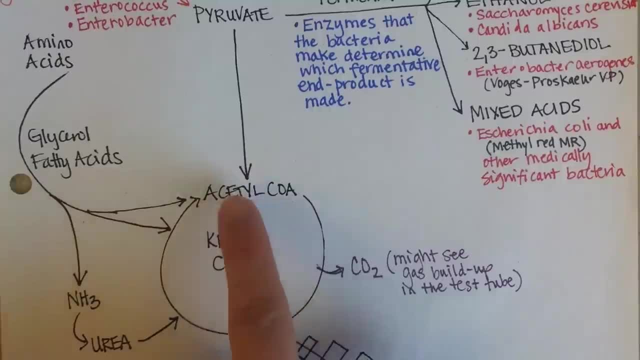 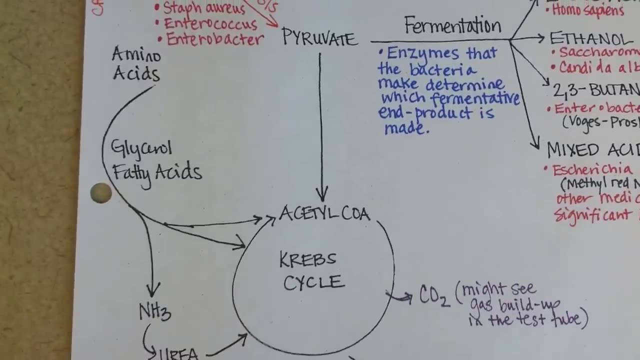 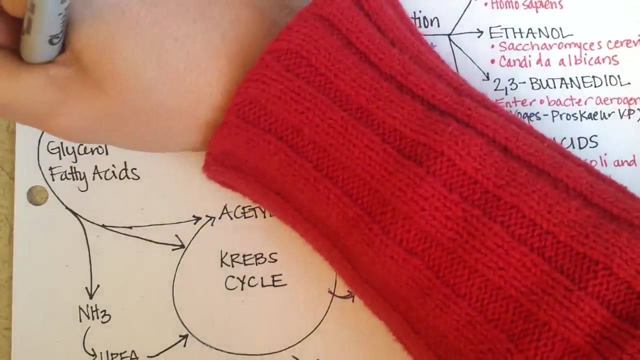 So pyruvate can enter this. but do you see all these other arrows? What you can see also going on is that fats and proteins can be used to make ATP. So over here we'll use a blue pen and you can write protein. 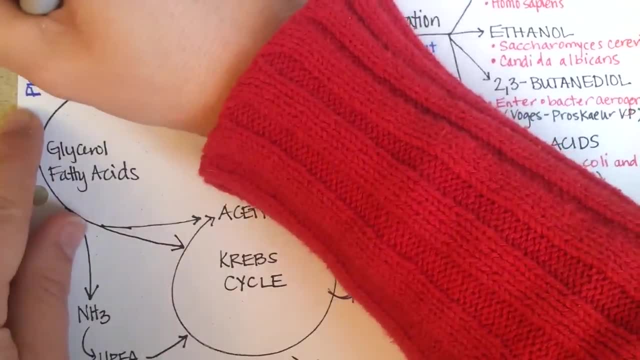 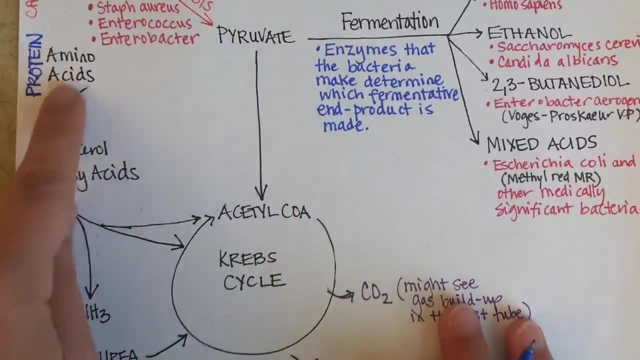 next to amino acids. So amino acids can- some of them can be converted into pyruvate and some of them can be converted into middle products that then can go into the acetyl or the Krebs cycle, citric acid cycle. So 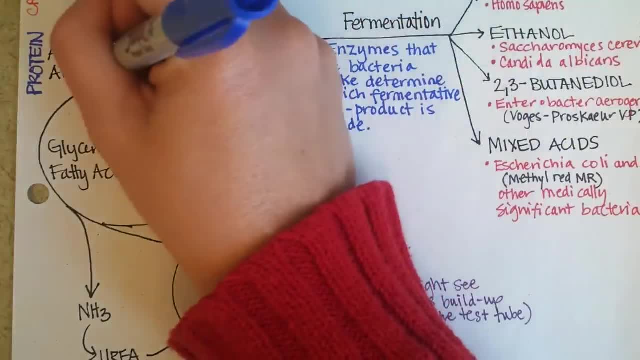 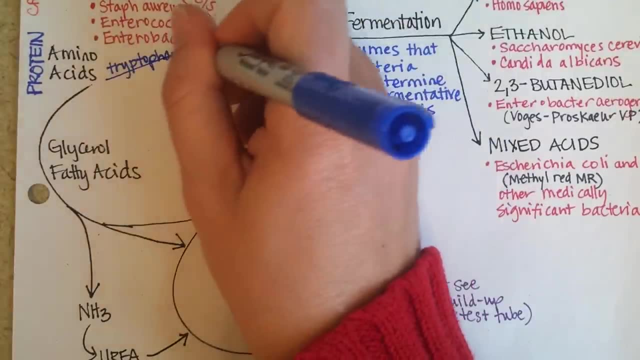 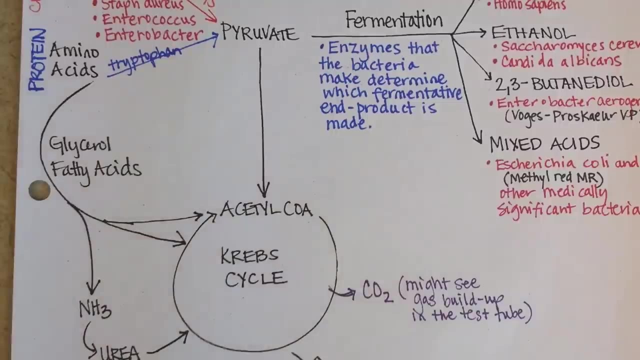 for example, tryptophan is an amino acid- one of the 20, that can be converted into pyruvate. Now there's a test that you can do, where you test for indole, And indole is a byproduct of tryptophan being. 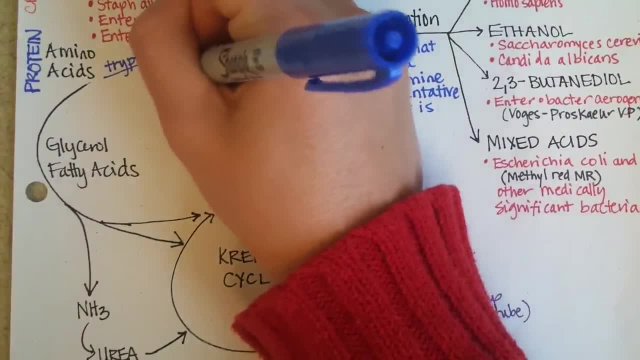 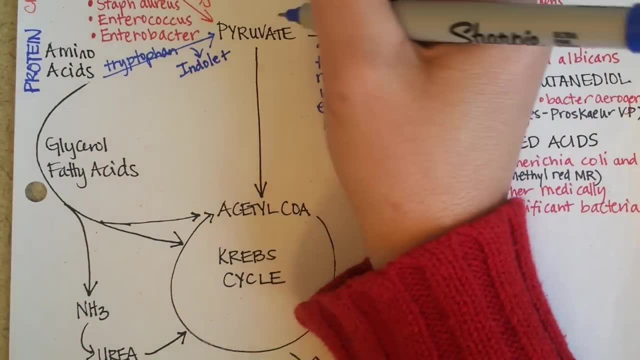 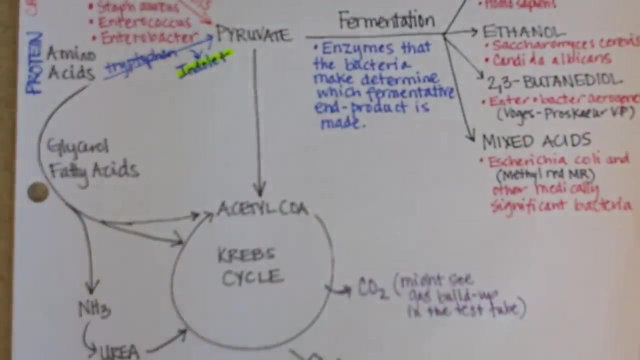 converted into pyruvate. So this bacteria- if, for example, if it was able to convert tryptophan to pyruvate, would test indole positive in the lab. And some bacteria are able to convert cysteine into. 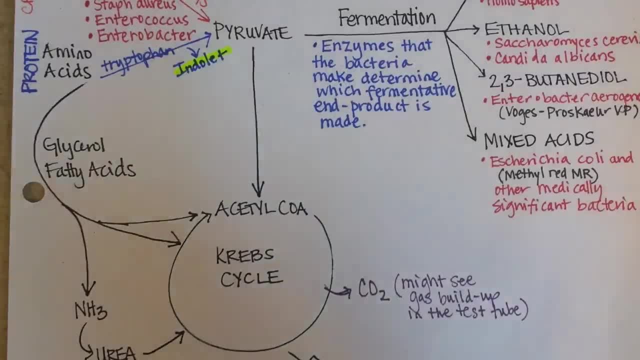 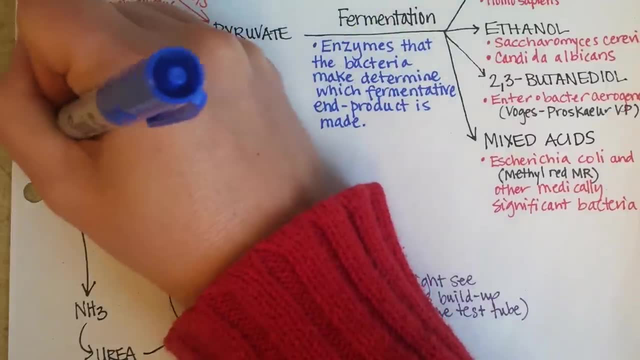 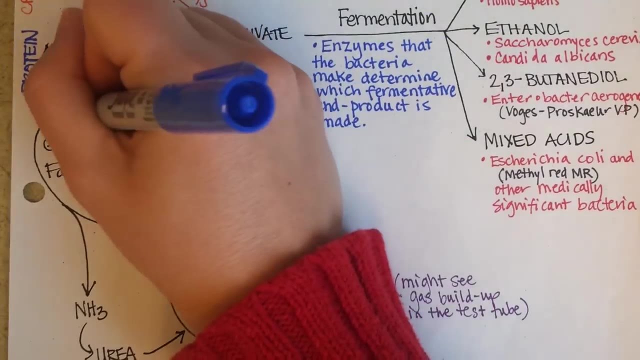 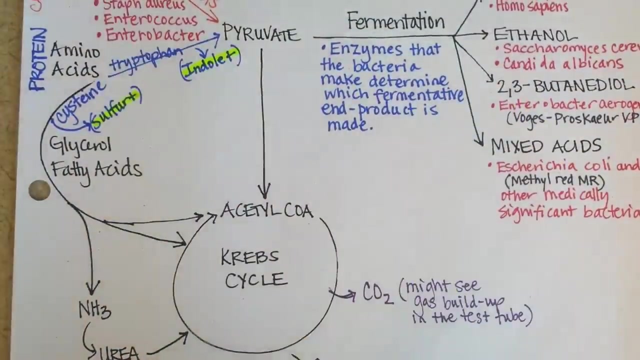 a product that can then go into the Krebs cycle. So you can write cysteine here And if that's the case, then sulfur is given off as a byproduct and this bacteria would be sulfur positive. Then you can use your blue highlighter. 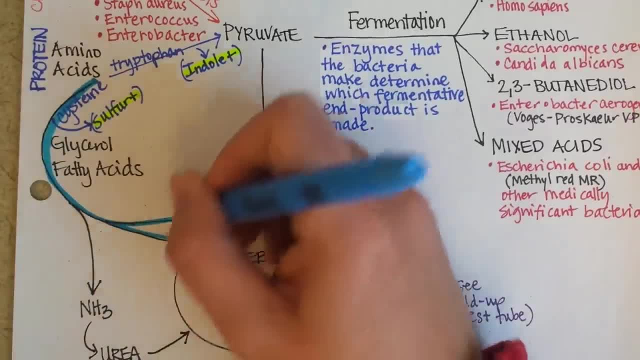 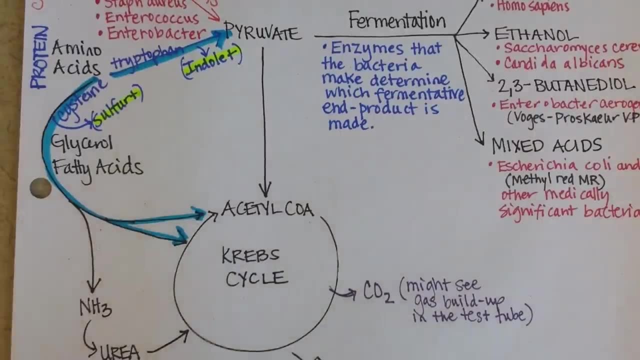 So some amino acids can be converted into acetyl-CoA or other products. Tryptophan can be converted straight into pyruvate. So the point is is that you know there are 20 different amino acids. 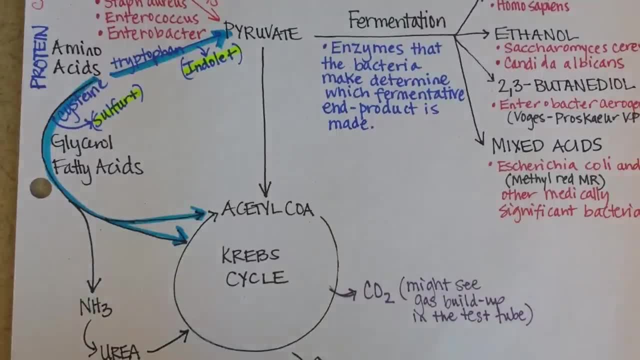 and there are different ways that those amino acids can be used to gather ATP for the cell. And what we're concerned about on this page is saying, okay, the bacteria that we're interested in, lab. what are some tests that we run that are looking at these different 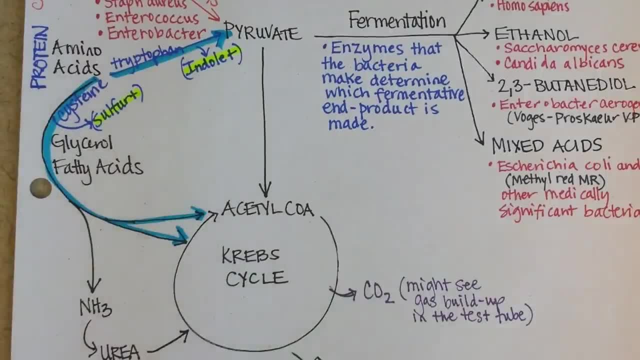 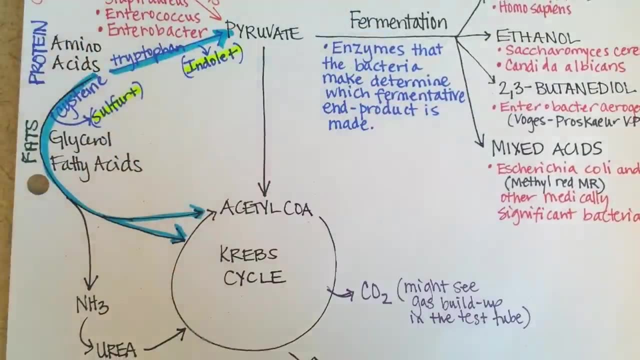 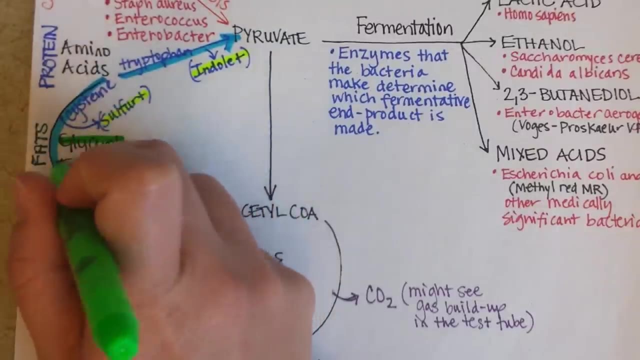 amino acid metabolic pathways. Fats can also be used to make ATP. I'm going to write that in a green pen. And when a triglyceride is broken down, it's broken down into a glycerol and then some fatty acid tails. 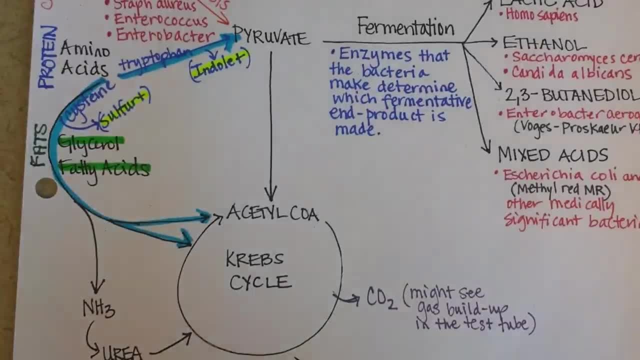 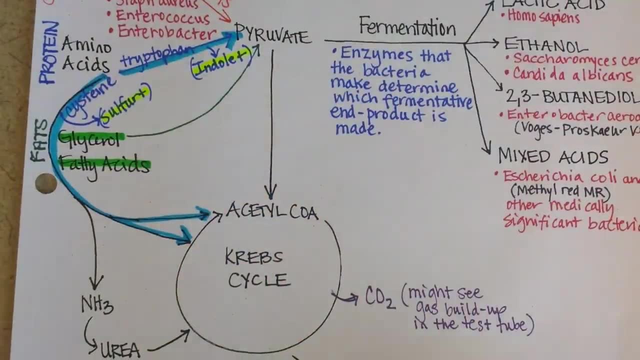 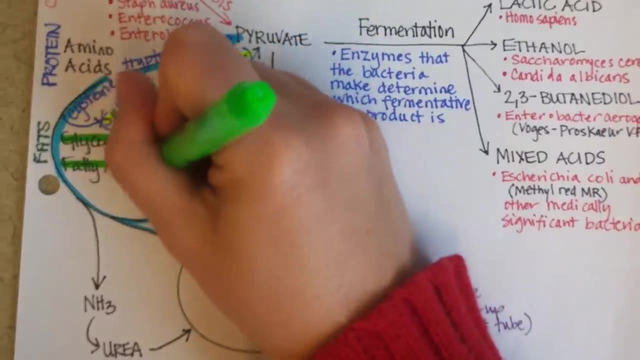 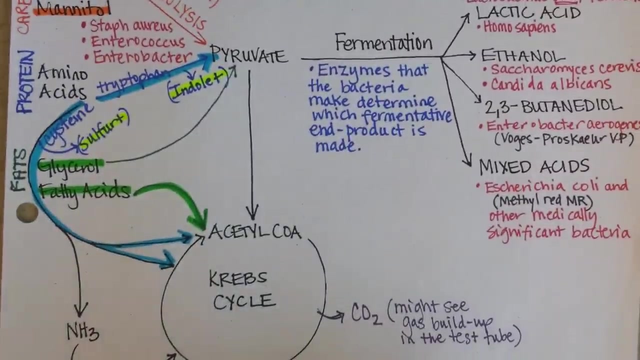 And those have different places to go. Glycerol is converted into pyruvate and fatty acids, head straight into the Krebs cycle. The point is is that bacteria, just like humans, can use a lot of different kinds of nutrients to make ATP. 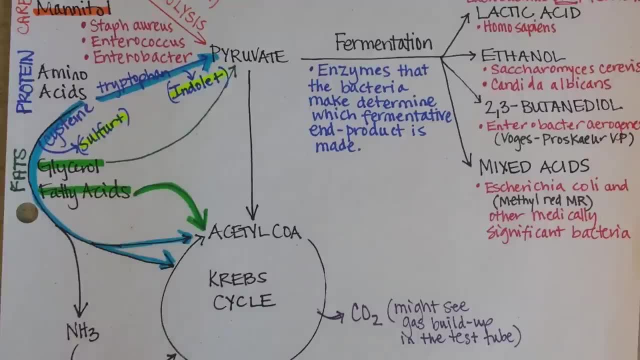 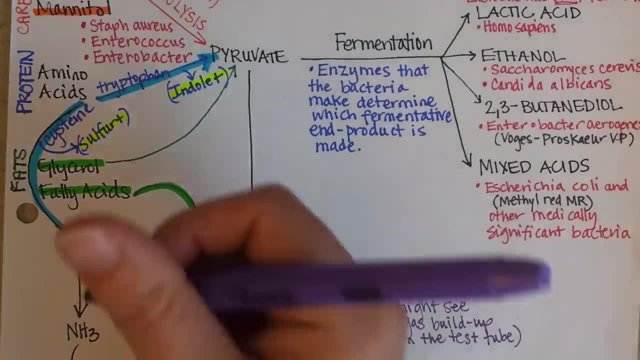 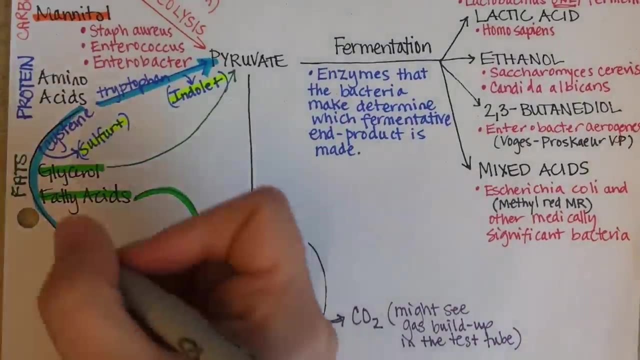 Okay now, if bacteria are going to use amino acids to try and make ATP, they have to deaminate them, And that's what this line represents. They have to take the amine group or the ammonia off of it. 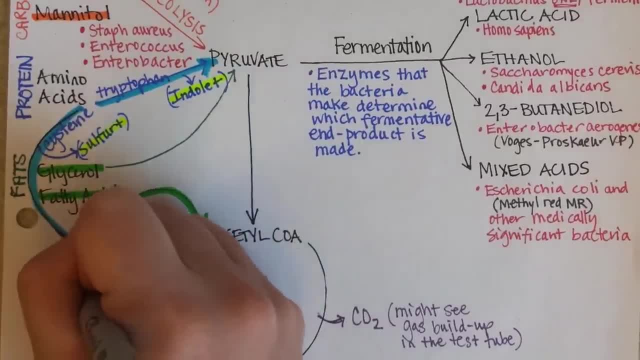 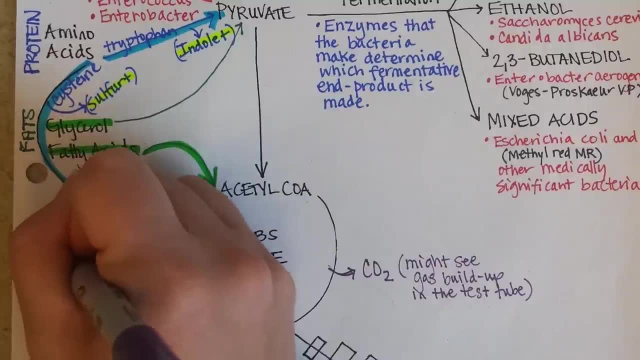 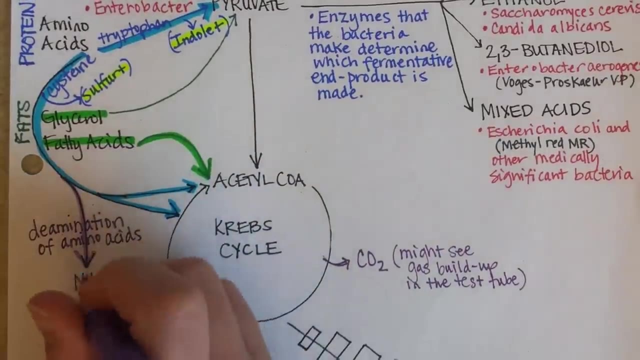 We have to do this too, Not just bacteria. So you have to deaminate an amino acid if you want to get ATP out of it, And what you're left with is a toxic byproduct called ammonia. Now, in humans, ammonia is converted into urea in the liver. 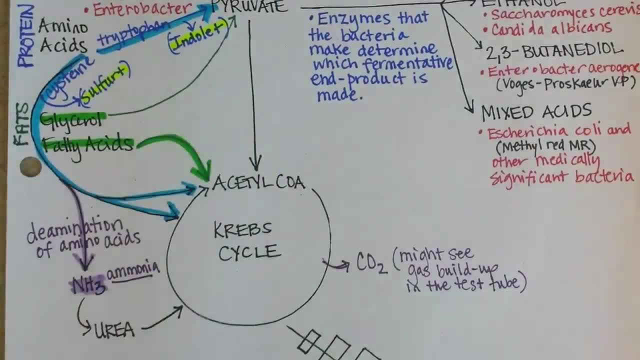 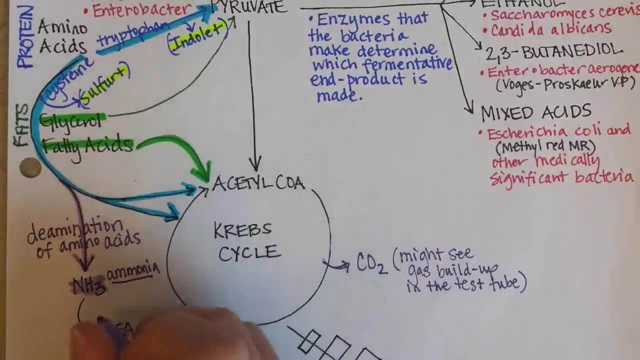 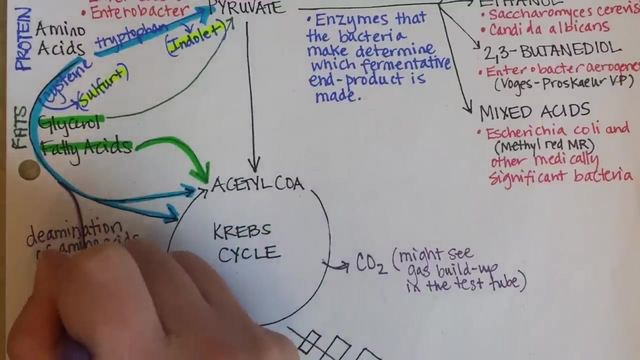 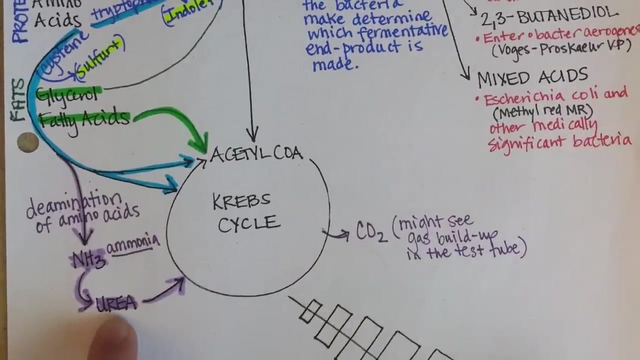 In bacteria, they can just excrete it, But some bacteria, like proteus, are actually able to take urea and use urea to make ATP again, So it's a very efficient process. Like in humans, urea is just a waste product. 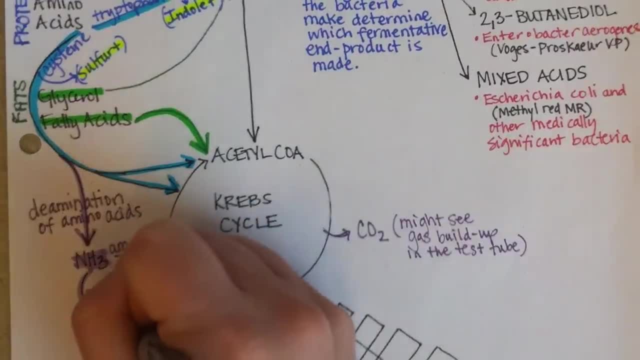 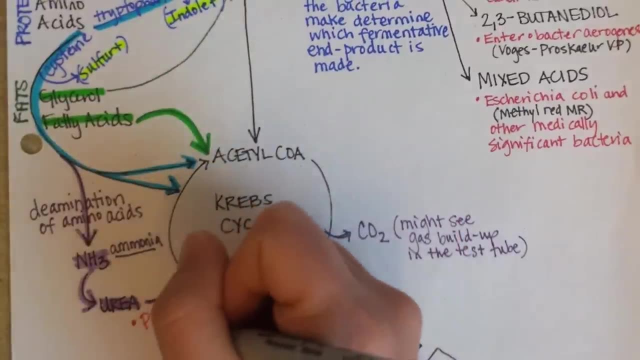 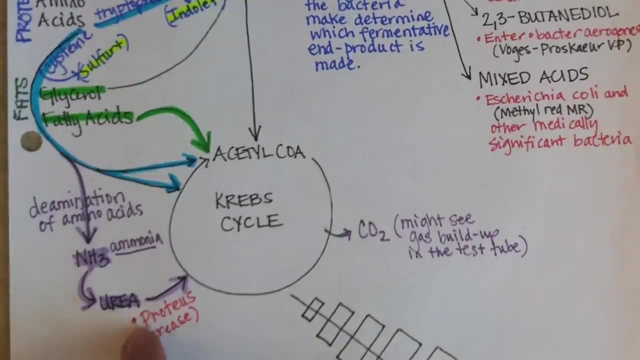 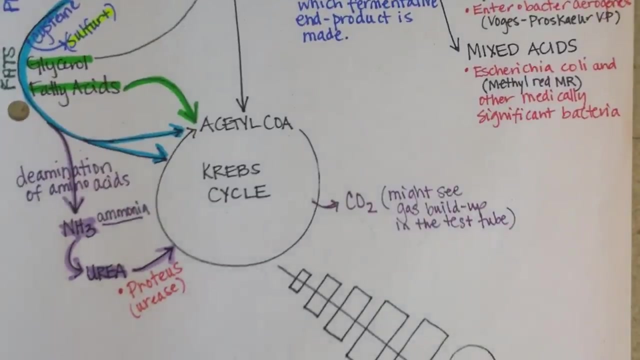 For proteus. urea is a food because it has an enzyme called urease, So it's able to use what would be a waste product. put it back into the Krebs cycle. get a little bit of ATP from it. Okay, now after the Krebs cycle. 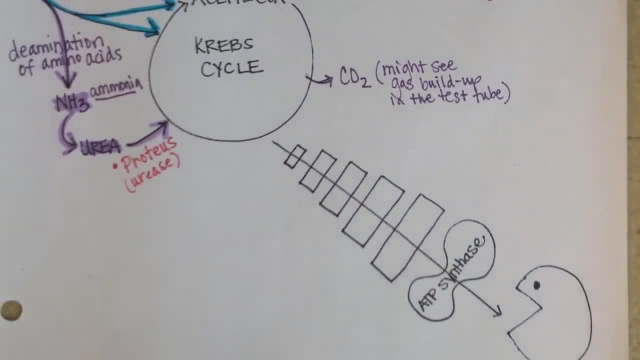 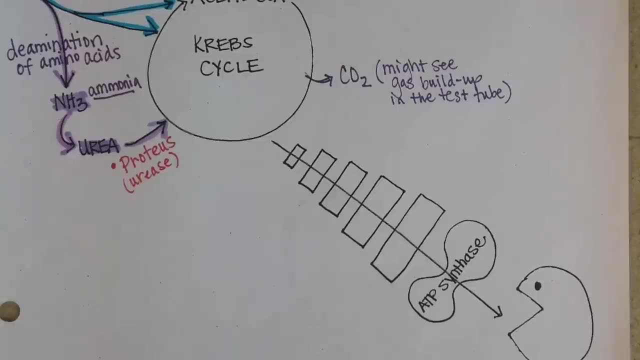 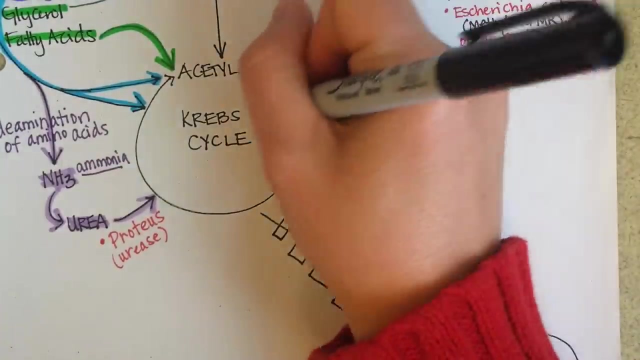 electrons from the amino acids, or electrons from the fatty acids, or electrons from the pyruvate- you know originally what was the carbohydrates. electrons from the nutrients are then going to be passed down. So if you were going to say what goes on in the Krebs cycle, 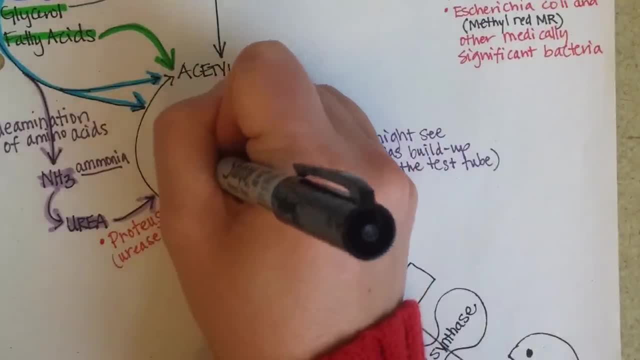 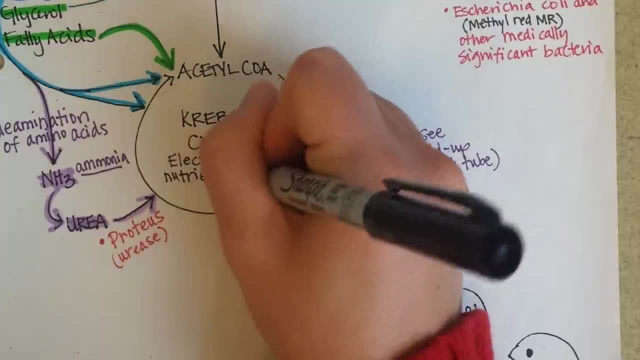 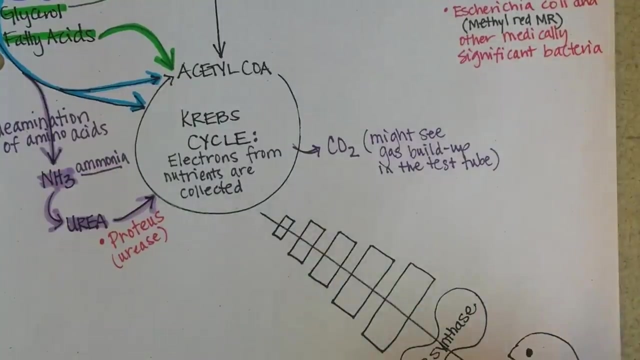 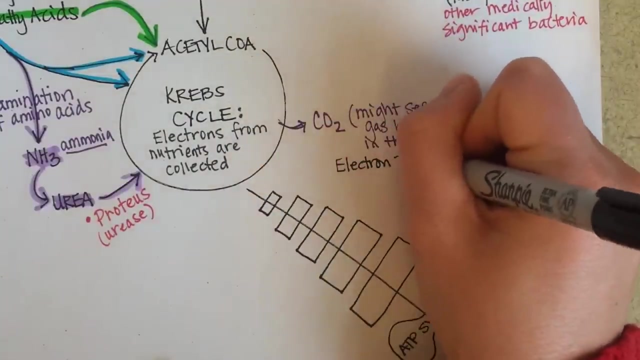 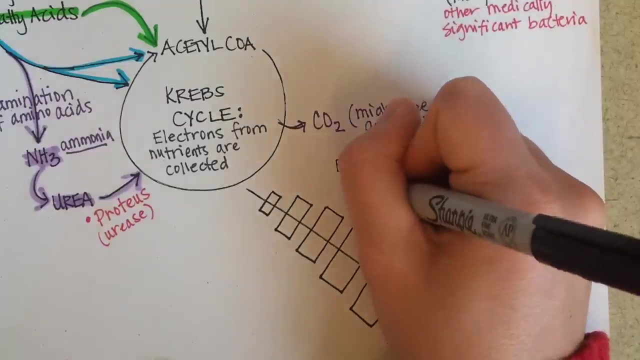 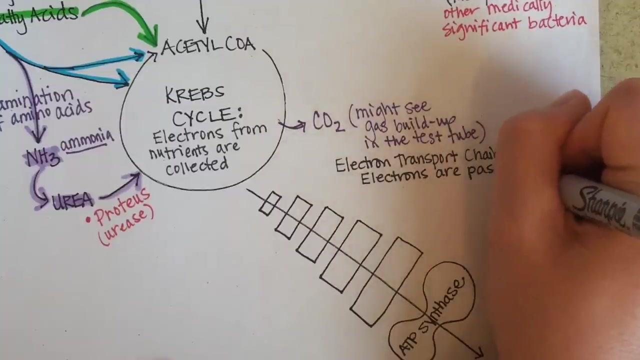 you could put electrons from the nutrients are collected And then, if you were going to say what goes on in the electron transport chain, right here you can put electrons from the proteins, electrons, electrons, electrons, and the energy from those electrons is used to make. 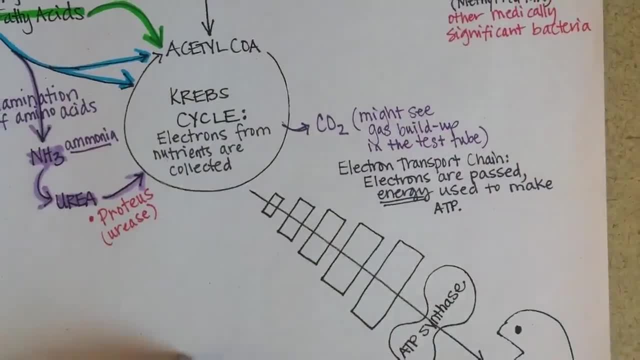 ATP. Okay, I'm going to take a look at the next step, a break, and then in the next video I'll finish this up.